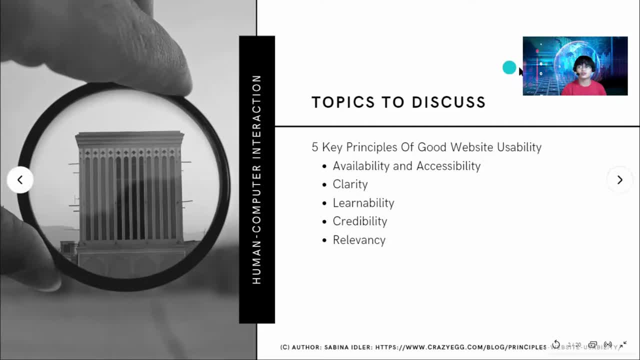 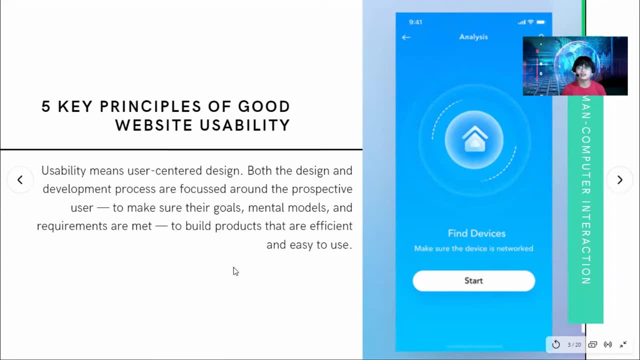 really great content, okay, so let's continue. okay, so what is usability? Usability means user-centered design. both. both the design and development process are focused around the prospective user to make sure their goals, mental models and requirements are met to build products that are efficient and easy to use. so it's very important that you should know this. different principles in 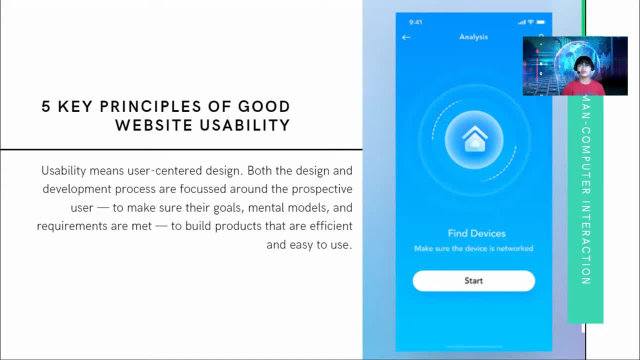 order for you to have a really great HSAI design, okay. so again, when we say usability, it means user-centered design. okay, you must know what are your goals, why you have the kind of design I think I can move this in here. okay, in order for you to build products that are efficient to efficient and easy to use. okay. 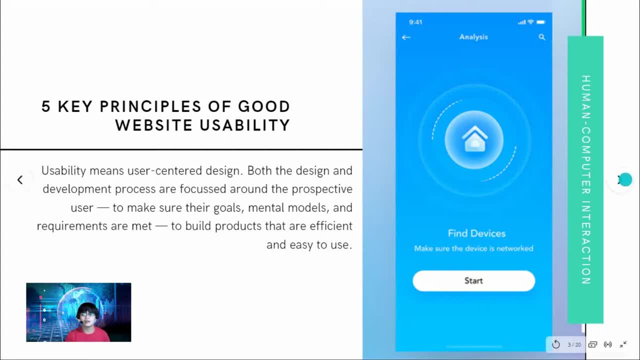 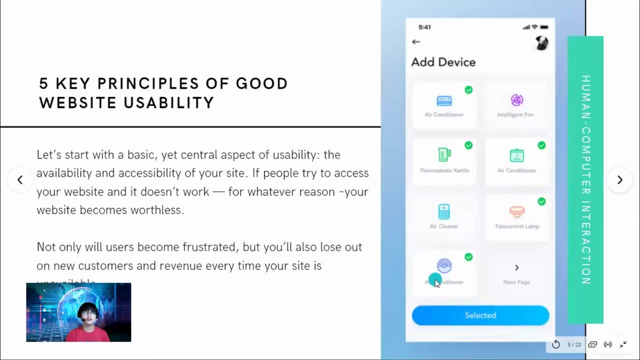 next. okay, first we have the availability and accessibility. okay, let's bring this back here. I think so. let's start with the basic yet central aspect of usability: the availability and accessibility of your site or of your application. so, if people try to access of your website or your application, 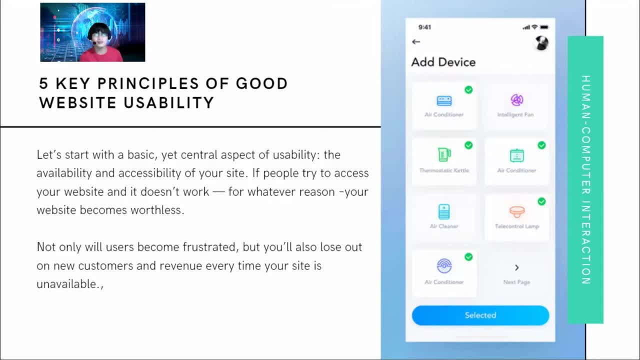 and it doesn't work, for whatever reason. your website becomes worthless or your application becomes worthless. okay, imagine you have this really great design, really great application, but when the user access it, then it gets down right. how would you feel? same as what you are experiencing in other? 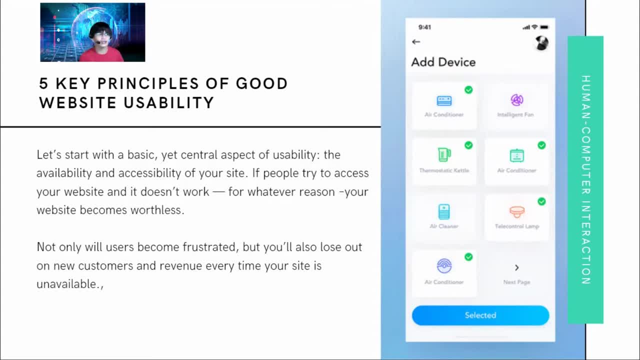 applications right, you feel frustrated and you feel like you don't like the application. it gets down, something like that. so not only will users become frustrated, but you also lose on new customers and revenue every time you use your site or your application. you also lose on new customers and revenue every time you use your site or your application. 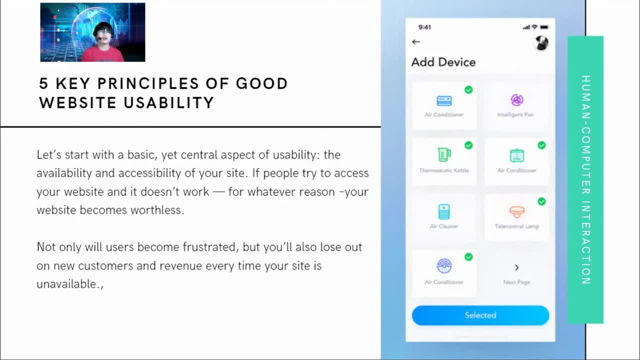 your site is unavailable. so imagine your application is all about an e-commerce, now an e-commerce- you, you sell online. but then one day now and of course you lose customers and driven you if you download the application. so it's very important that it's always up. 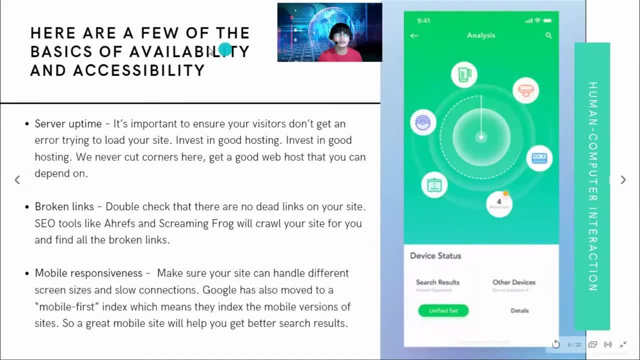 okay, so these are the different basic availability and accessibility. server uptime: okay, so the server of time. it's very important to ensure your visitors don't get into error trying to load your application, trying to load your site, so invest in a good hosting, invest in a good hosting. so invest in a good hosting. so invest in a good hosting. 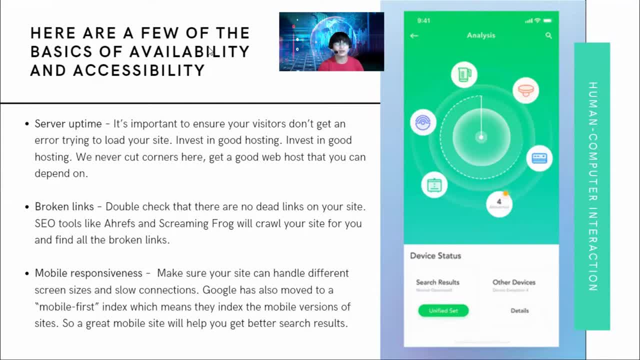 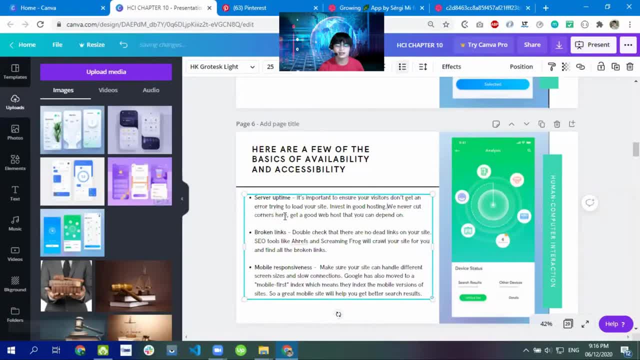 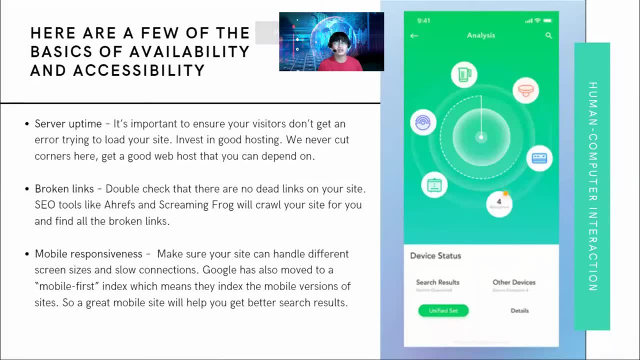 um, yes, let me correct this one. um, yes, let me correct this one. sorry about that, sorry about that. sorry about that. okay, sorry, okay. invest in a good thing: we never cut okay. invest in a good thing- we never cut. okay. invest in a good thing: we never cut corners here. get a good web host. 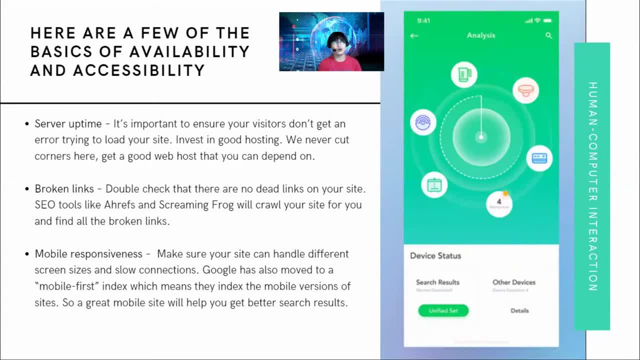 corners here, get a good web host. corners here: get a good web host that you can depend on. so when you are that you can depend on, so when you are that you can depend on, so when you are putting your application into live, putting your application into live, 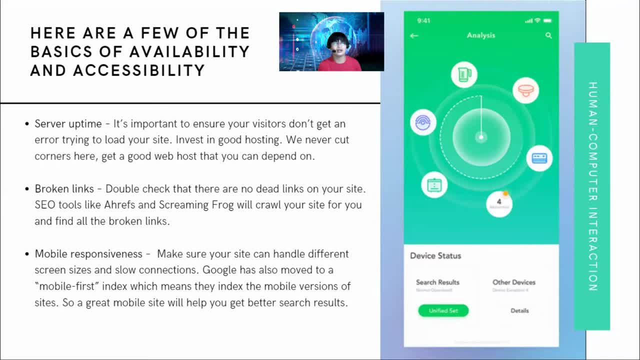 putting your application into live system system system. you should have a really, you should have a really, you should have a really great, great, great namanga hosting services. but don't worry namanga hosting services, but don't worry namanga hosting services, but don't worry because 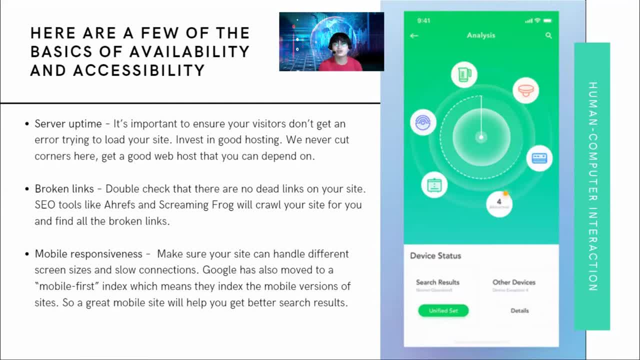 because, because they're gonna call you uh different good, they're gonna call you uh different good. they're gonna call you uh different good. hosting providers that you can hosting, providers that you can hosting, providers that you can look into and then check if. look into and then check if. 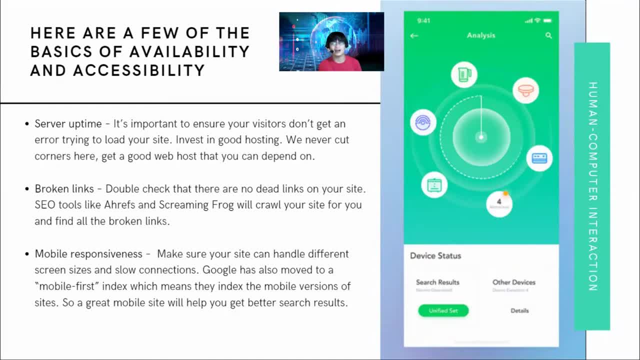 look into and then check if asaang imo need and asaang must better. asaang imo need and asaang must better. asaang imo need and asaang must better and not nila. okay and not nila okay. 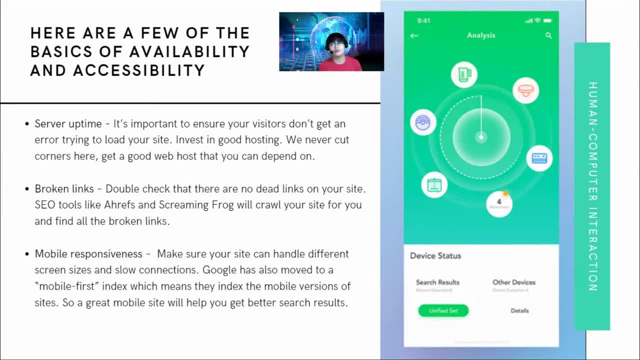 and not nila. okay, there are a lot of uh hosting, uh, there are a lot of uh hosting, uh, there are a lot of uh hosting uh web hosting services, and then web hosting services, and then web hosting services and then cheaper up with any young prices, okay. 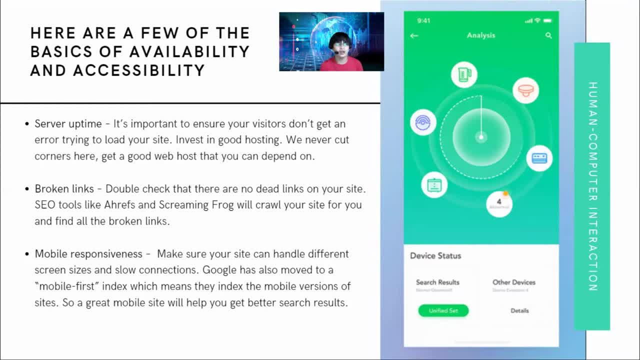 cheaper up with any young prices- okay, cheaper up with any young prices, okay, so so. so it's to ensure that it's to ensure that it's to ensure that your visitors don't get an error trying your visitors don't get an error trying your visitors don't get an error trying to load your application. 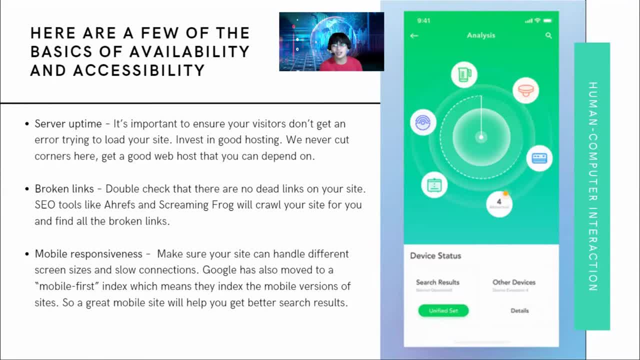 to load your application. to load your application. next, broken links. so it's very important. next, broken links. so it's very important. next, broken links. so it's very important that your application does not have any, that your application does not have any, that your application does not have any broken links. because imagine if a user 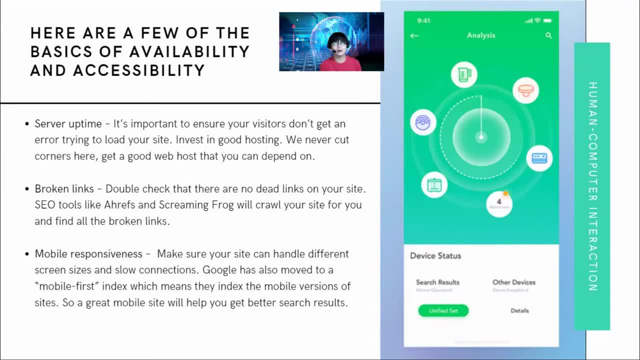 broken links, because imagine if a user broken links, because imagine if a user, and then i try to access something, and then i try to access something, and then i try to access something and then, um, i try to access some link and then i try to access some link. 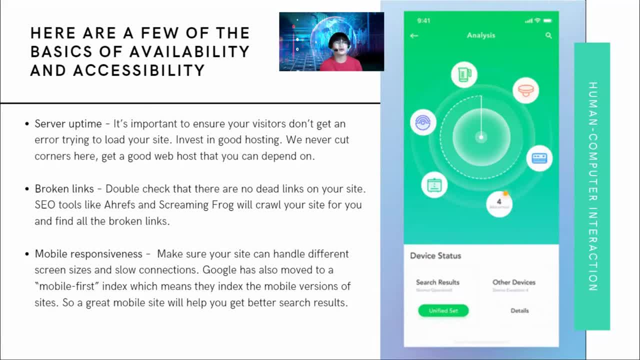 and then i try to access some link, but click now, error die will additionally. but click now, error die will additionally. but click now, error die will additionally exist, exist, exist. so double check that there are noted. so double check that there are noted. so double check that there are noted. links on your. 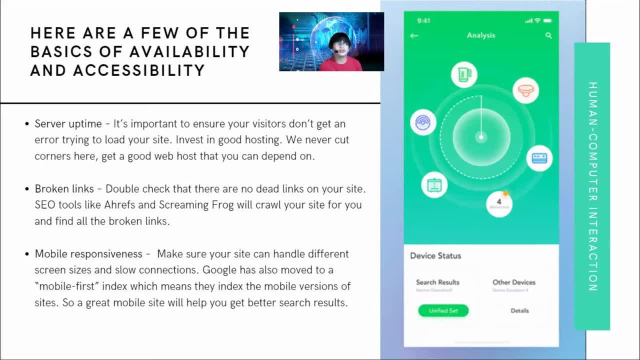 links on your links on your sap or application. so is a tools. is a sap or application. so is a tools. is a sap or application. so is a tools. is a tools like tools, like tools like ahrefs and screaming frog will crawl. ahrefs and screaming frog will crawl. 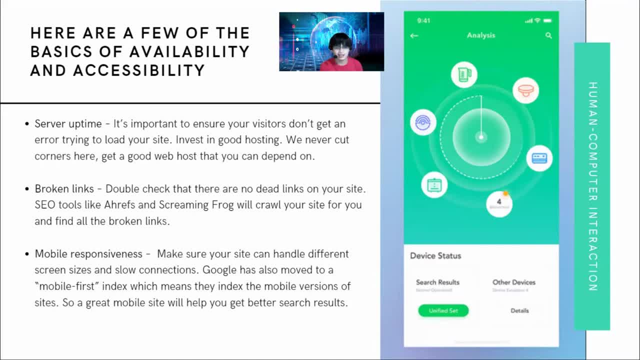 ahrefs and screaming frog will crawl your side for you, your side for you, your side for you, and find all the broken links. okay so, and find all the broken links, okay so, and find all the broken links, okay so. you can use this. you can use this. 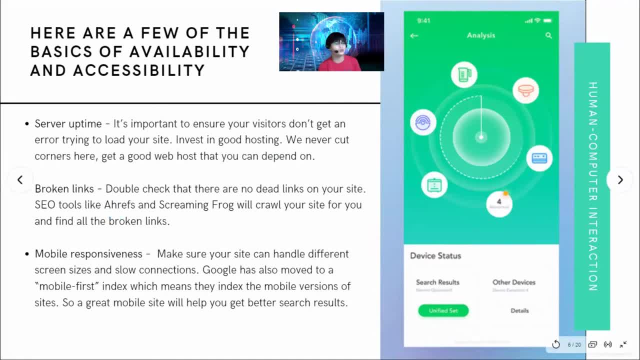 you can use this tools um install on national tools. tools um install on national tools. tools. um install on national tools. ahrefs and screaming frog. then that ahrefs and screaming frog, then that ahrefs and screaming frog, then that tool. we're gonna find the link. 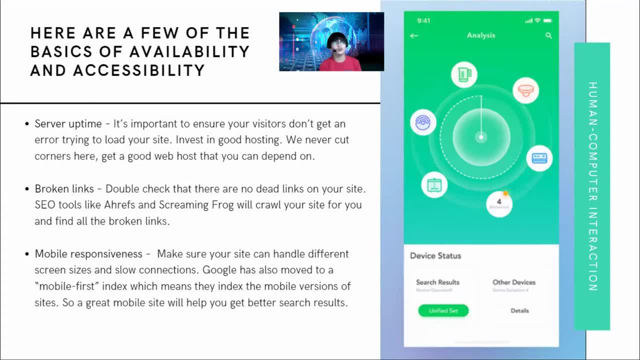 tool, we're gonna find the link tool, we're gonna find the link in the broken same application, in the broken same application, in the broken same application. so, after finding this broken link, a. so after finding this broken link, a. so after finding this broken link, a button is, of course, to fix it. 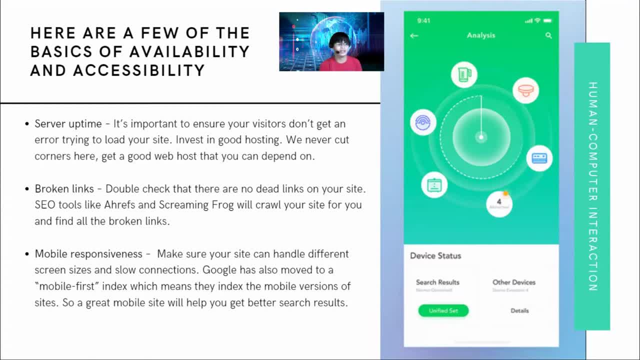 button is, of course, to fix it. button is, of course, to fix it. same codes, same codes, same codes, broken links, broken links, broken links. next, next, next, mobile responsiveness. okay, so, as of the mobile responsiveness. okay, so, as of the mobile responsiveness. okay, so, as of the moment, as, as you may have noticed, 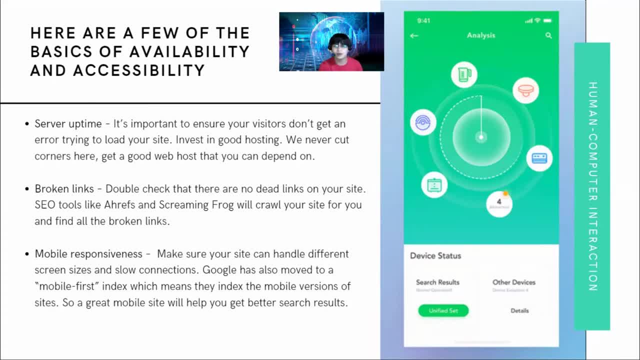 moment as, as you may have noticed, moment as, as you may have noticed, everyone know a lot of us is now using, everyone know a lot of us is now using, everyone know a lot of us is now using cell phones, cell phones, cell phones, smartphones, mobile devices. so it's very 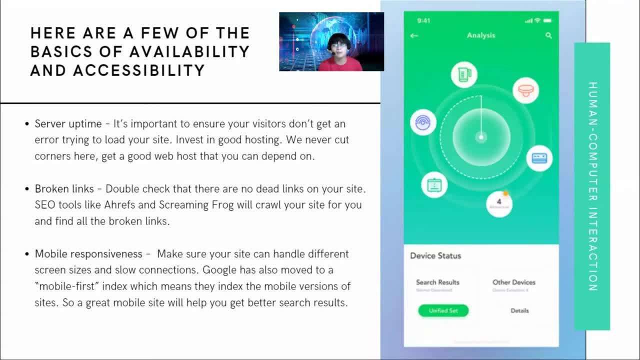 smartphones, mobile devices. so it's very smartphones, mobile devices. so it's very important that your application, important that your application, important that your application must be um mobile responsive, must be um mobile responsive, must be um mobile responsive, must be very viewable same one phone. must be very viewable same one phone. 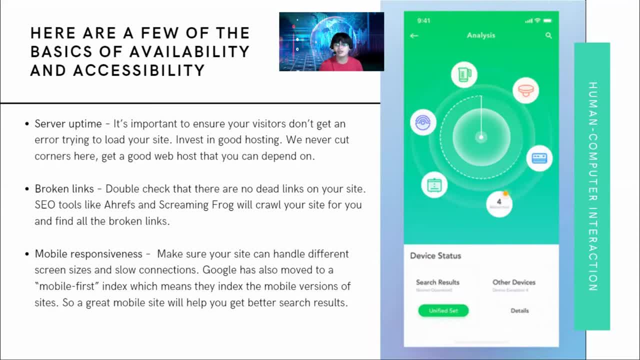 must be very viewable. same one phone. okay, so make sure your site can handle. okay, so make sure your site can handle. okay, so make sure your site can handle. different screen, different screen, different screen sizes and slow connections. google sizes and slow connections. google sizes and slow connections. google has also moved to a mobile first. 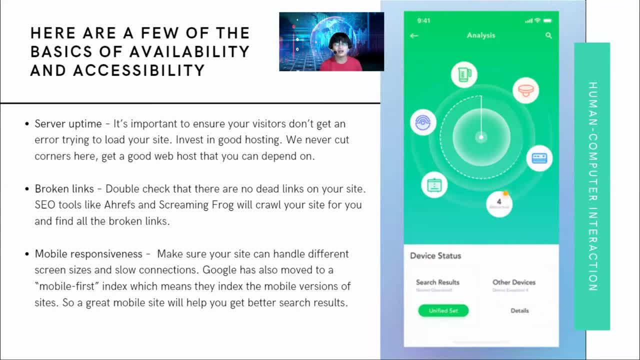 has also moved to a mobile first, has also moved to a mobile first index, which means if they index the index, which means if they index the index, which means if they index the mobile versions of the site, mobile versions of the site, mobile versions of the site. so a great mobile site will help you get. 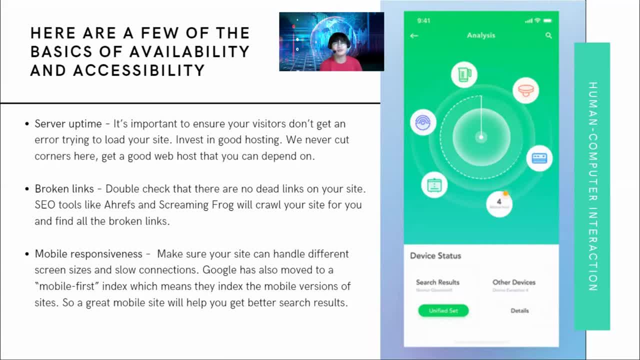 so a great mobile site will help you get, so a great mobile site will help you get better search results, better search results, better search results. okay, okay, okay. not all of us has you know laptops. not all of us has you know laptops. not all of us has you know laptops, desktops, computers. 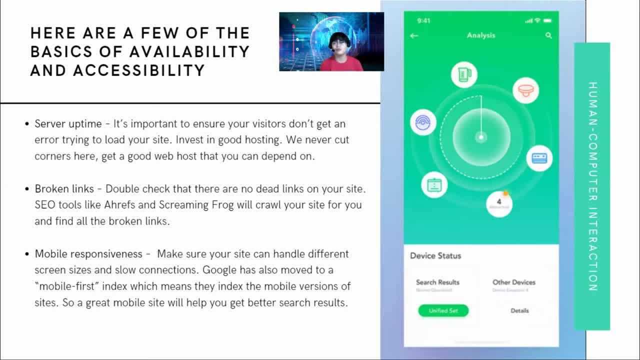 desktops, computers, desktops, computers. a lot of us is using only mobile, so it's a lot of us is using only mobile, so it's a lot of us is using only mobile. so it's very important that your application is very important that your application is. 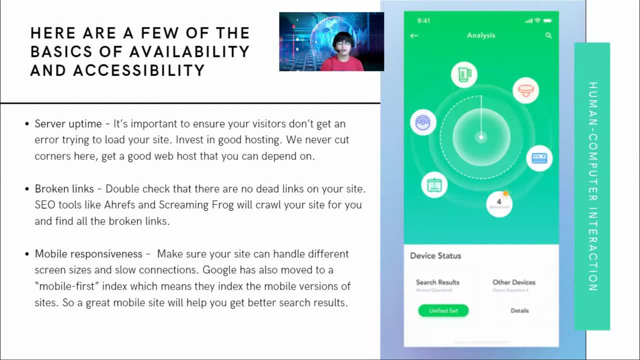 very important that your application is a mobile friendly, mobile responsive, a mobile friendly, mobile responsive, a mobile friendly, mobile responsive. i hope you guys can still hear my voice. i hope you guys can still hear my voice. i hope you guys can still hear my voice clearly because, clearly, because. 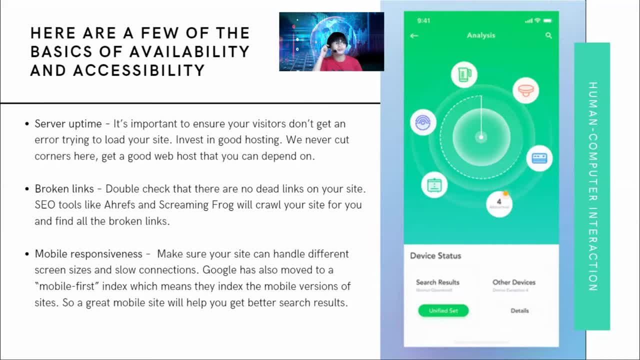 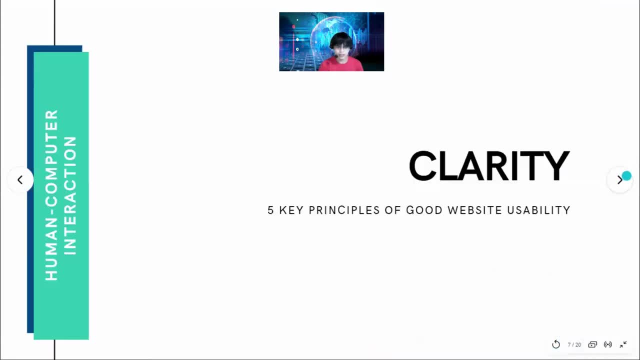 clearly, because it's raining so hard in here, but it's raining so hard in here, but it's raining so hard in here. but yeah, i hope number don't get me up on call. i hope number don't get me up on call. i hope number don't get me up on call. okay, so that's one, the accessibility. 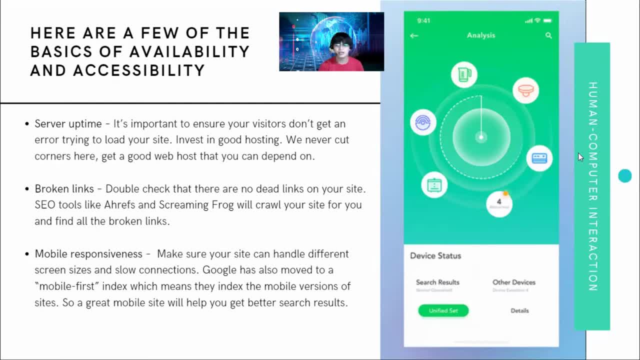 okay, so that's one. the accessibility. okay, so that's one: the accessibility, and and and um availability. next we have um availability. next we have um availability. next we have the clarity of course. uh, it's a the clarity of course. uh, it's a the clarity of course. uh, it's a self-explanatory clarity. 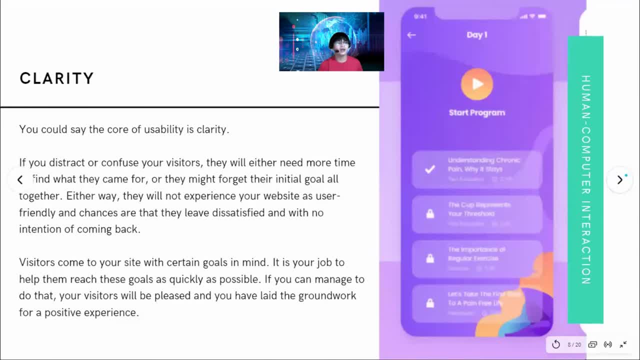 self-explanatory clarity. self-explanatory clarity: um, um, um. you can say the core of usability is. you can say the core of usability is. you can say the core of usability is clarity. so if you distract or confuse clarity. so if you distract or confuse. 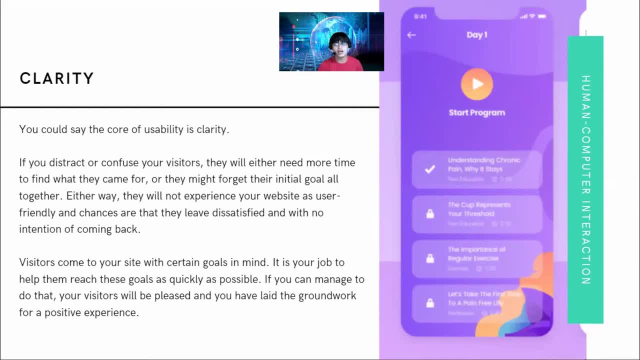 clarity. so if you distract or confuse your visitors, your visitors, your visitors, they will neither need more time to find, they will neither need more time to find, they will neither need more time to find what they came for, what they came for what they came for, or they might forget their initial goal. 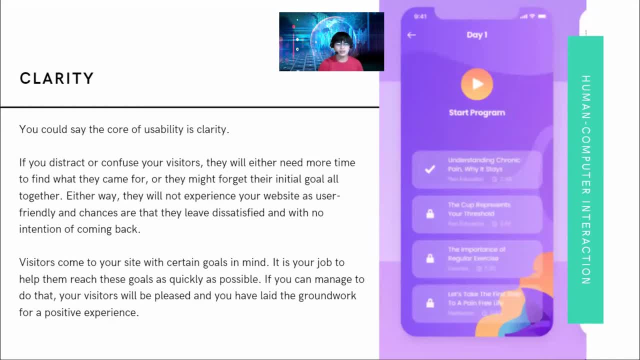 or they might forget their initial goal, or they might forget their initial goal all together, so either way. all together, so either way. all together, so either way, they will not experience your website, as they will not experience your website, as they will not experience your website as a user friendly and chances that 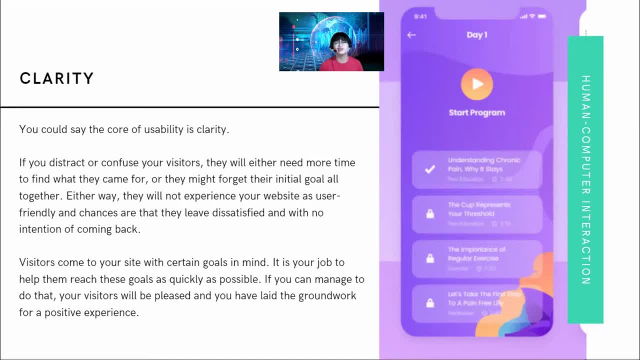 a user friendly and chances that a user friendly- and chances that are are are they live dissatisfied and with no, they live dissatisfied and with no, they live dissatisfied and with no intention of coming back. intention of coming back. intention of coming back so visitors come to your side with a 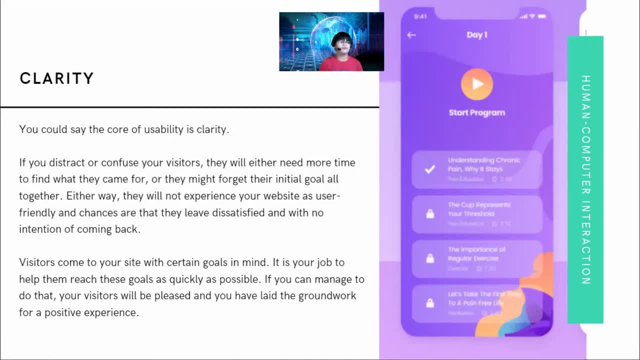 so visitors come to your side with a. so visitors come to your side with a certain goals in mind, certain goals in mind, certain goals in mind. it is your job to help them reach these. it is your job to help them reach these. it is your job to help them reach these goals as quickly as possible. so, if you 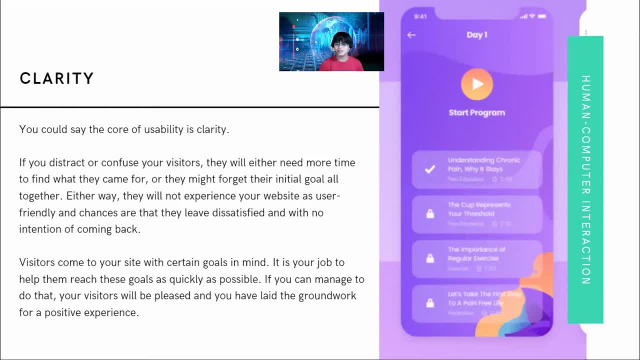 goals as quickly as possible. so if you goals as quickly as possible, so if you can manage to do that, can manage to do that, can manage to do that, your visitors will be pleased and you, your visitors, will be pleased, and you, your visitors, will be pleased and you have laid the groundwork for positive. 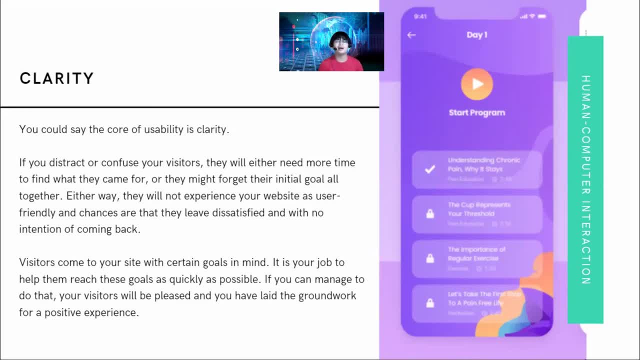 have laid the groundwork for positive, have laid the groundwork for positive experience. experience if i am the user, if i'm going to go to the dashboard, okay, okay. for example, i have this online application, oh, um, an e-commerce application, sorry guys, it's okay. so, uh, let me post this one. 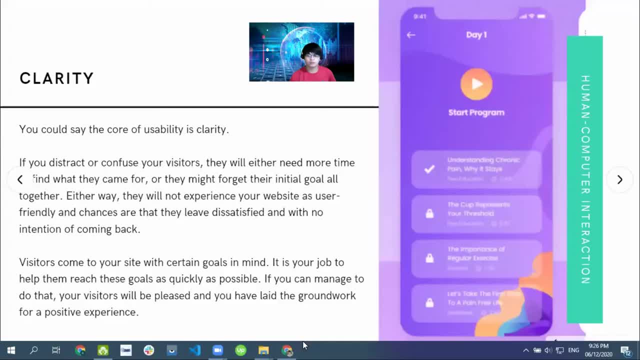 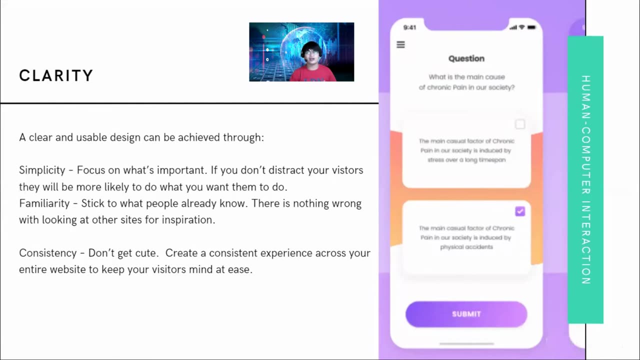 i think we can continue now, so let's move on to the next slide. okay, so clarity, so a clear and usable design can be achieved through first, simplicity. okay, it must be simple as possible. focus on what's important. if you don't distract your visitors, they will. 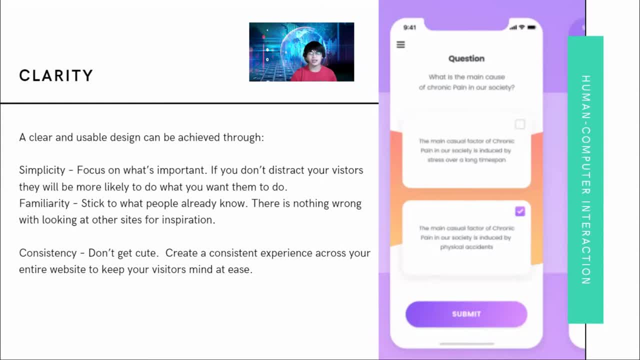 be more likely to do what you want them to do. and then familiarity. so stick to what people already know. there is nothing wrong with looking at the other sites for inspiration. okay, that's why i'm i'm telling you to, um, find some other applications out there and make it as an. 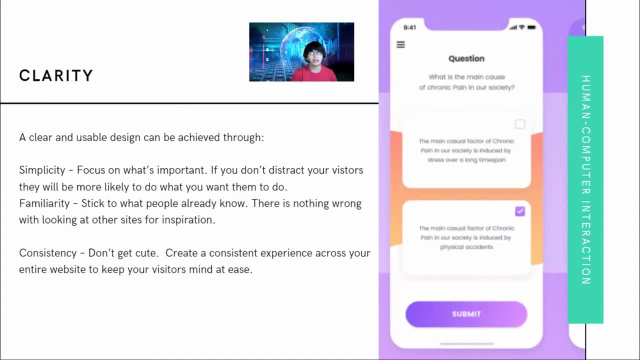 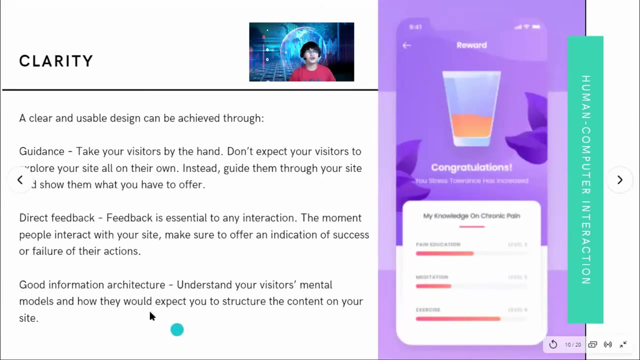 inspiration. and next is consistency. don't get cute, okay, so create a consistent experience across your entire website to keep your visitor's mind at ease. okay so, okay, okay, so additional. now i know another for you to achieve usable design is guidance. take your visitors by the hand. don't expect your visitors to explore your site all on their own. instead, 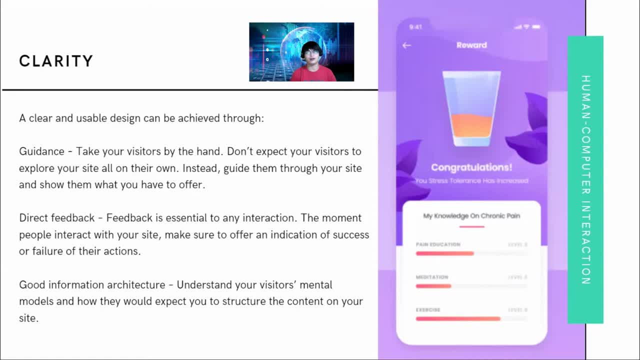 guide them through your site and show them what you have to offer, and direct feedback. so feedback is essential to any interaction. the moment people interact with your site, make sure to offer an indication of success or failure of their actions, so especially when the user entered an invalid. 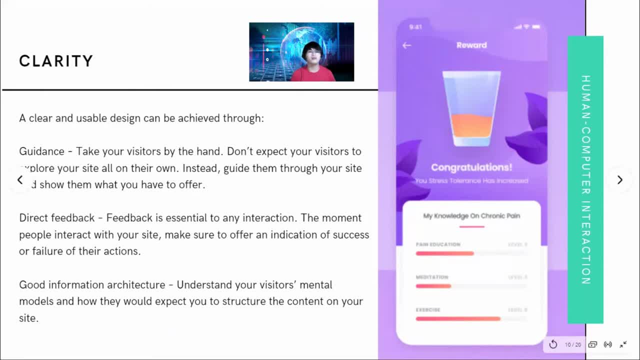 email. so it is very important to make sure that the users understand what you are doing and it is very important to have the same feedback. okay, and then good information architecture. so understand your visitors mental models and how they would expect you to structure the content of your application. that's it. I guess that's it. so that's clarity. you should have clarity, okay. 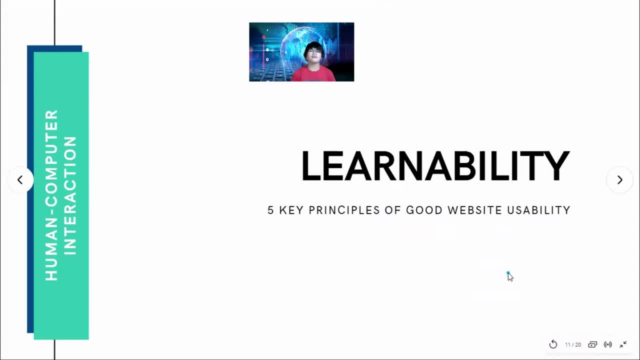 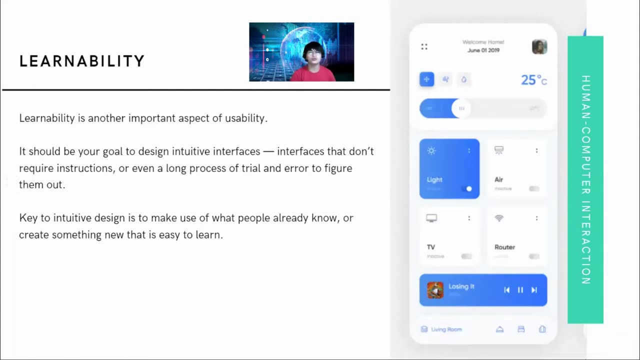 let's move on to the third one. we have learnability- okay, so easy to think about terms, no, and self-explanatory, okay. so when we say learnability, um, it should be your goal to design intuitive interfaces, interfaces that don't require instructions or even a long process of trial and error to figure. 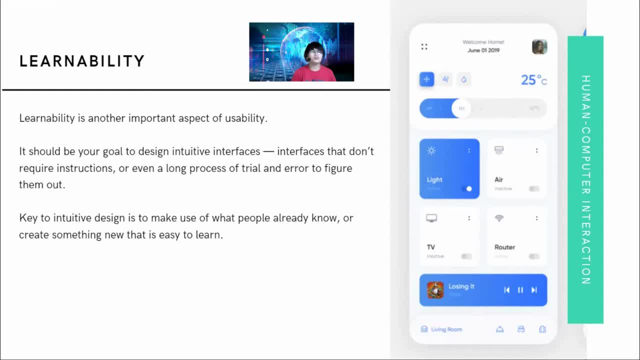 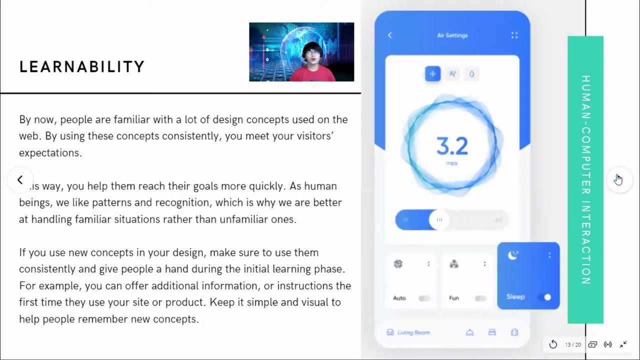 them out. so, okay, to end of the design is to make sure make use of what people already know or create something new that is easy to learn. okay, so, as as what you have observed, even next, okay, so by now people are familiar with a lot of design concepts used on, yes, in the web or 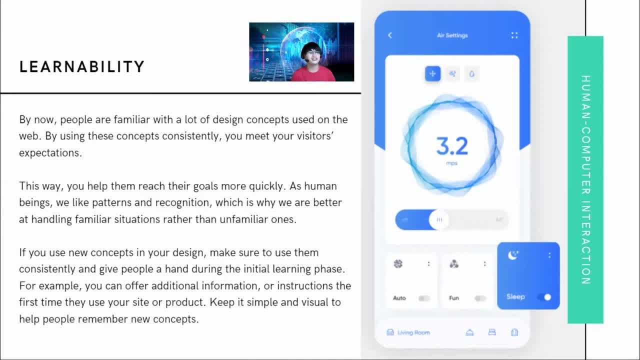 in a mobile. so by using these concepts consistently, you meet your visitors expectations, so this way, you help them reach their goal more quickly. so, as human being, we like patterns and recognitions, which is why we are better at handling familiar situations rather than unfamiliar ones. let me check. 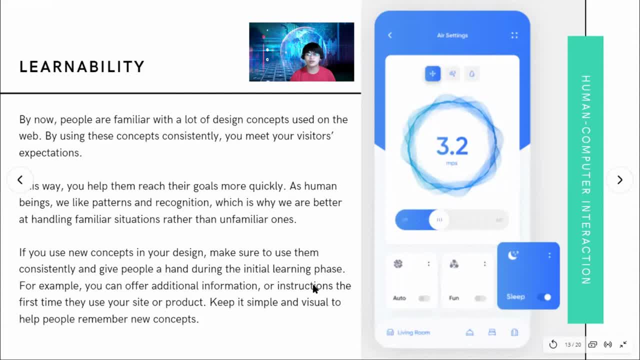 okay, it's recording. so if you use new concepts in your design, make sure to use them consistently and give people a hand during the initial learning phase so, for example, you can offer additional information or instructions the first time they use your site or product. keep it simple and visual to help people remember. you can set if you can remember. 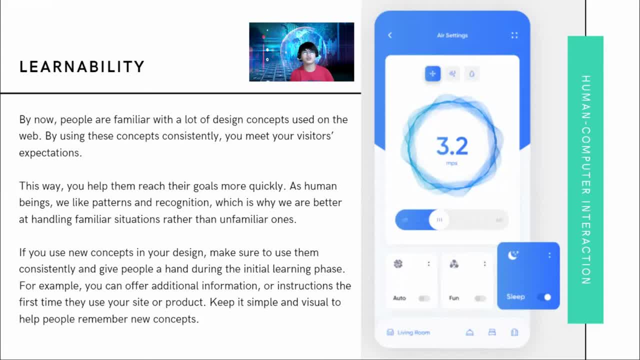 to open it. it looks like it's in a loop. so there is a tutorial? no, there is a tutorial if it can be used. so if your visitors need or need quick tutorials where they can find the toolbars, where they can find the menus for you to use, then it will be easier if you downloaded it. if your site is complicated, 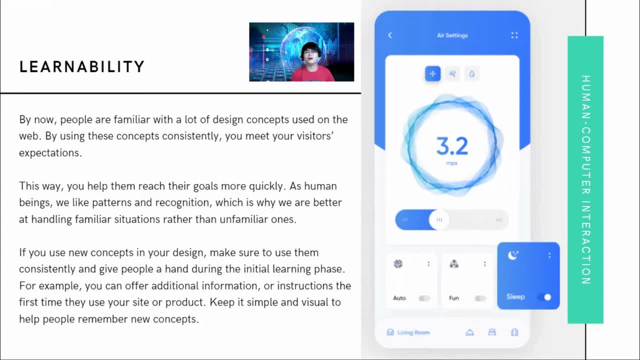 you can set the website, but it will be better if it's simple for you, because this is a simple website and it's a simple app, but if you are a professional user, you can have a website that is similar to yours. if you're a professional user, you can have a website that is similar to your website in a simple way. 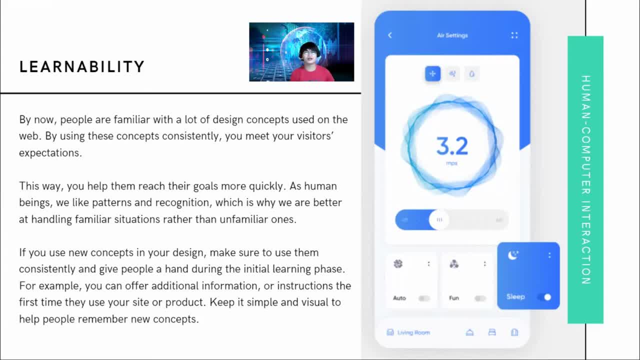 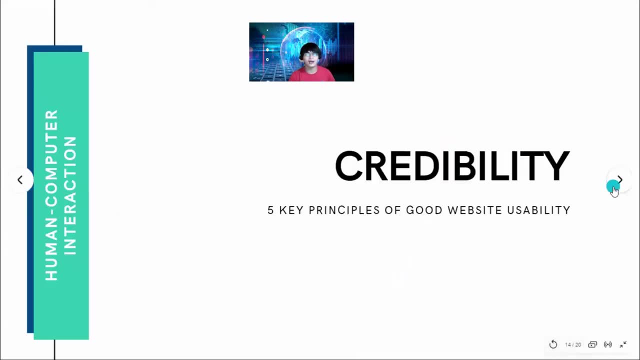 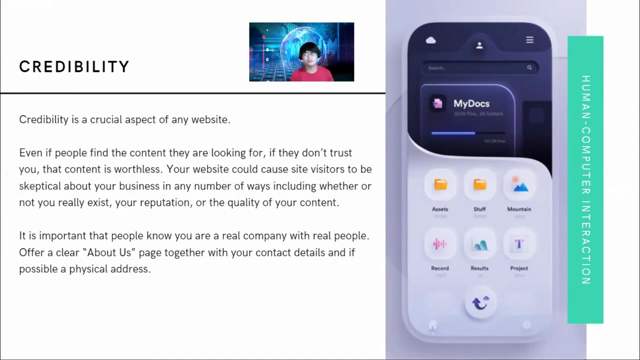 this is what we are going to discuss: clarity, learnability. let's proceed with the next one. we have credibility, very simple term, very self-explanatory. this is a very crucial aspect of any application. so, even if people find the content they are looking for, if they don't trust you? 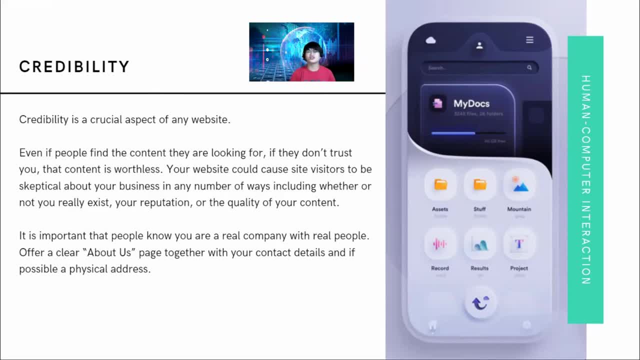 that content is worthless. so your website could cause site visitors to be skeptical about your business in any number of ways, including whether or not you really exist, your reputation or the quality of your content. is it true? is it a scammer system? sorry guys? application. 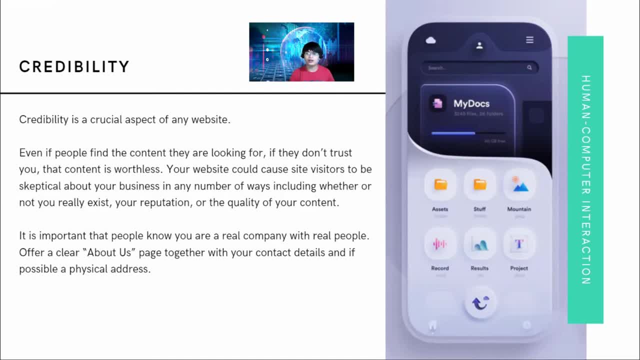 so it is very important that people know you are a real company with real people. offer a clear about us. you should put about us page, put different together with your contact details and, if possible, a physical address. if you can't see it, it is very bad if you put application. 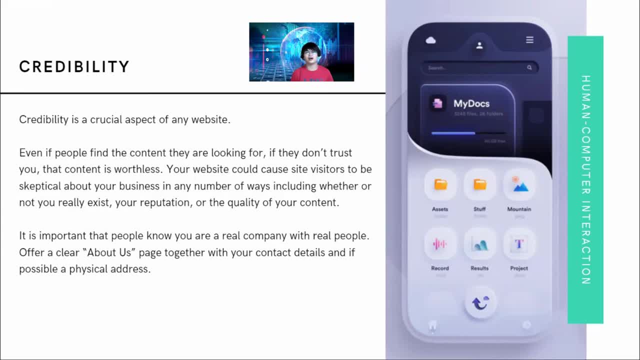 without a physical office. you can't see it. you can't see it. you can't see people with it, right? so you should put about us page. if you can't see it, okay, if you can't see the business, you should put about us page. 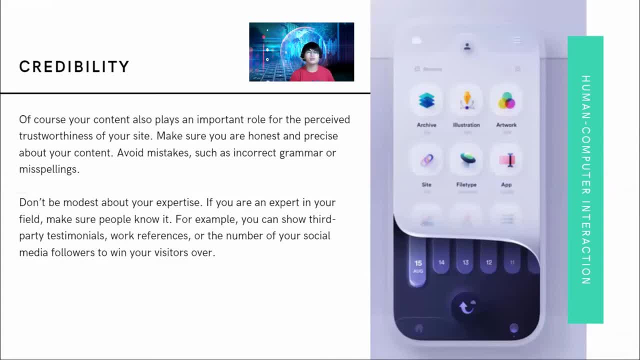 so, of course, your content also plays an important role for the perceived trustworthiness of your site. make sure you are honest and precise about your content. avoid mistakes such as incorrect grammar or misspellings. don't be modest about your expertise if you are an expert. 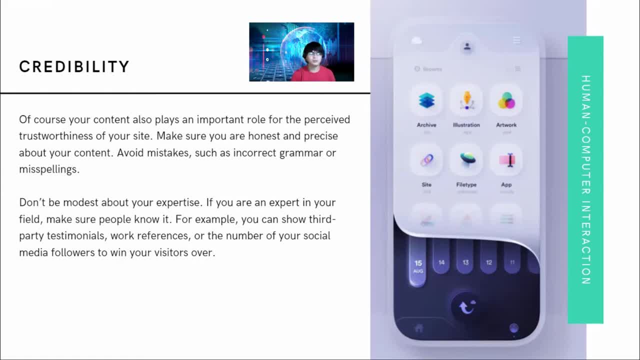 in your field, make sure people know about it. so, for example, you can show third party testimonials, work references or the number of social media followers to win your visitors, so that people can trust you, because there are different testimonials from other users that they have experienced while using this application. 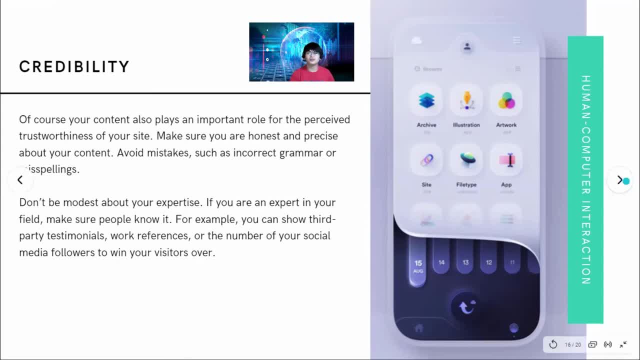 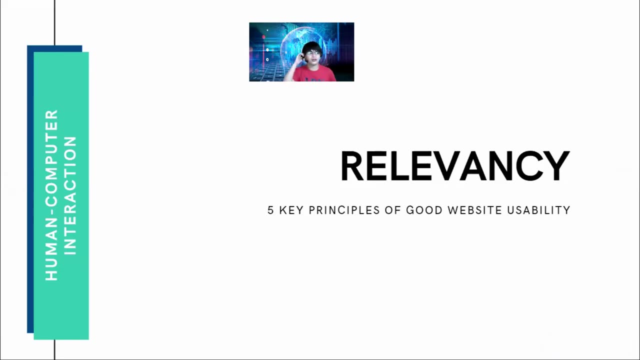 okay, it is very important for you to shop. if you change product, you take a look at the product list, the readings and then the testimonials so you can see if it is legit, if it is fake. so same as when doing or creating a system. next is relevancy. 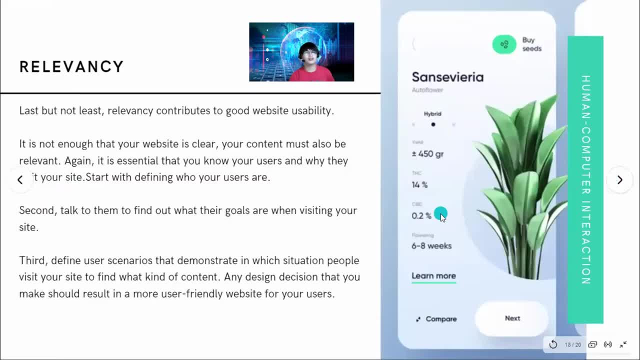 okay, relevancy. it is very important. this is the last but not least, okay, relevancy contributes to a good website visibility. so it is not enough that your website is clear. your content must also be relevant. okay, again, it is essential that you know your users and why they visit your site. 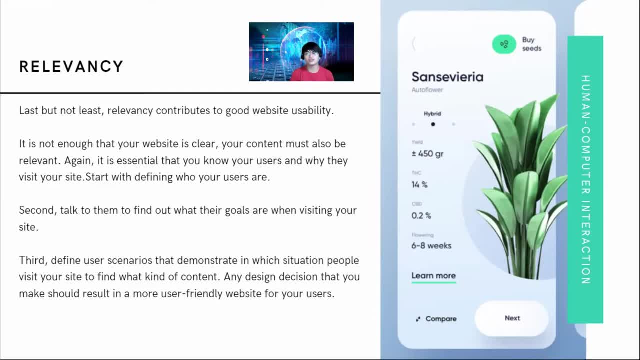 start with defining who your users are. you should know your users before designing an application. second, talk to them to find out what their goals are when visiting your site. okay, and the third one: define user scenarios that demonstrate in which situation people visit your site to find what kind of content. 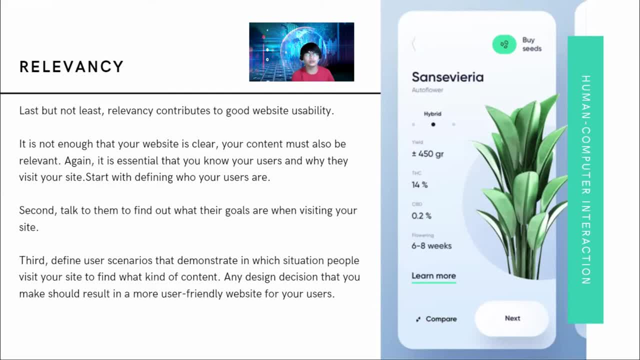 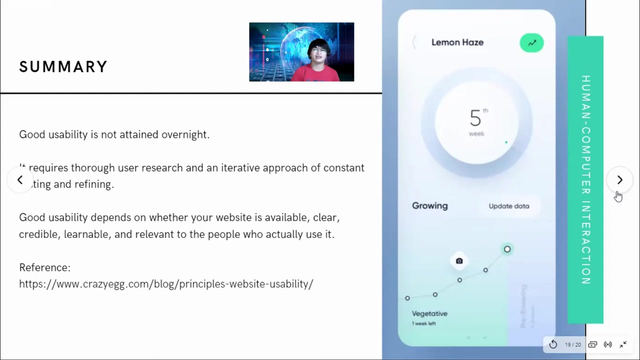 so any design decisions that you make should result in a more user-friendly website for your users. it should be complete, because if you just visited and nothing is complete, nothing that you can earn, then your application is complete. okay, so that's the last one. so, in summary,